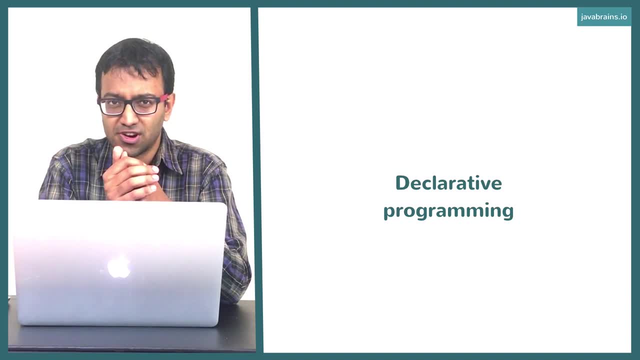 right. So you have some piece of text, you've written HTML code for it, right? You have your divs or paragraphs or whatever, and you want to center it. How do you do that? One way to do this is using imperative programming, where you're actually writing the steps to center the HTML. 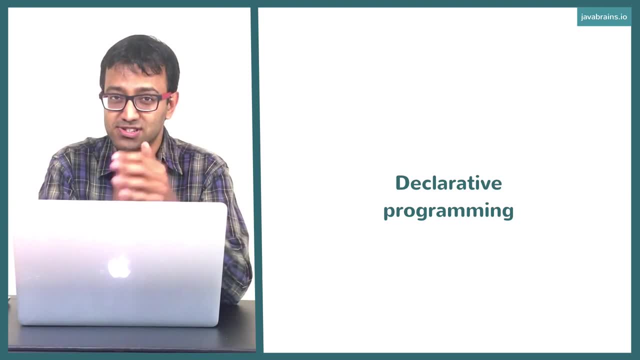 Right, You can say: okay, I'm going to figure out the width of the browser, right? Okay, this is the amount. I'm going to figure out the width of the HTML element that you need to center, which is a paragraph. right, I'm going to divide the width of the browser by two so that you get. 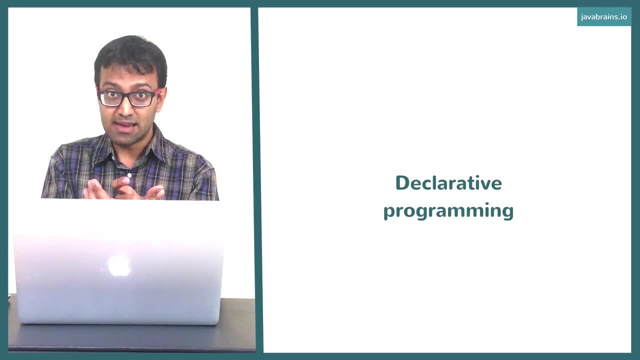 the exact middle. I'm going to divide the width of the paragraph by two, so you get the exact middle, and then I position the paragraph at the middle, offset by the half of the paragraph. Does that make sense? You're actually performing the steps to center an element in the middle, figuring out. 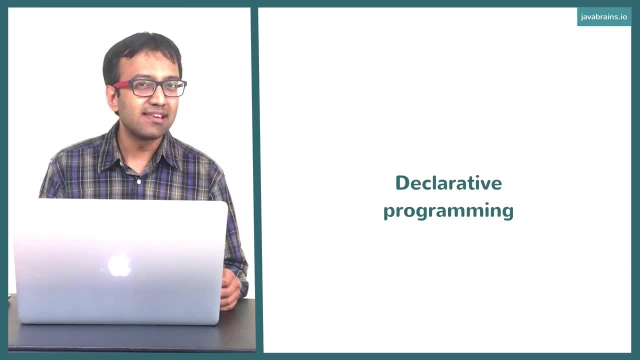 the dimensions, figuring out the center point and then centering that element. So that is imperative programming, But you don't do that in HTML. What you do in HTML is align colon center right. There's a CSS style that you apply, which is: you want the element centered right. So what you're doing 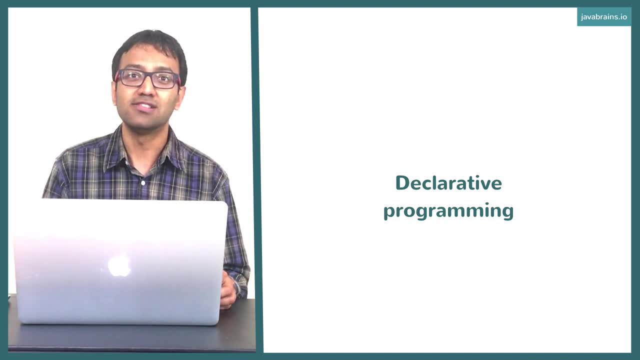 there is declarative programming. You're not imperatively preparing all the steps to center the paragraph. Somebody has already written the logic to center any element in the middle of the container. That's using CSS. All you're going to do is you're going to declare to the browser and say: 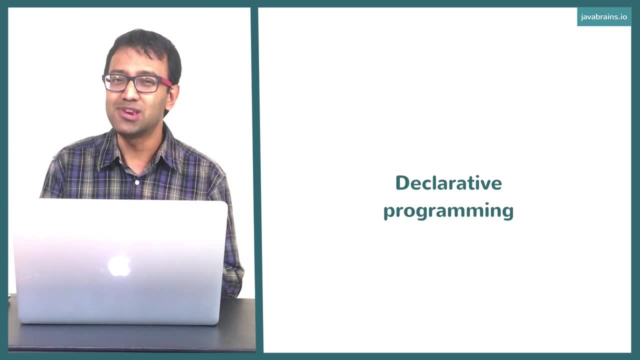 hey, browser, I need this element in the center. When you do that, you declare that by using align colon center and then the browser does the rest, because the browser has the logic that goes with that align center declaration. Browser already knows what to do when it sees that declaration. 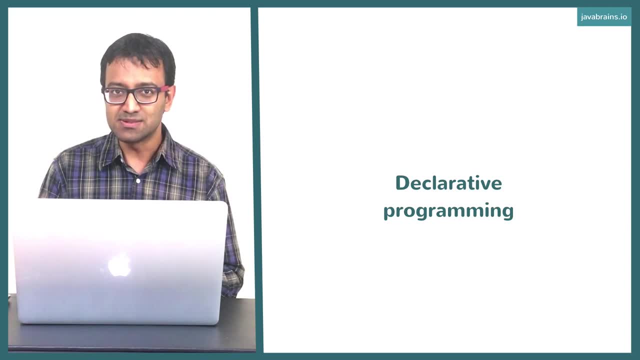 and it's going to do it for you, right? So this is the distinction between declarative and imperative. When you're coding in AngularJS, you're going to be doing a lot of declarative programming. You're not going to write the steps one by one. What you're going to do is create custom elements, create. 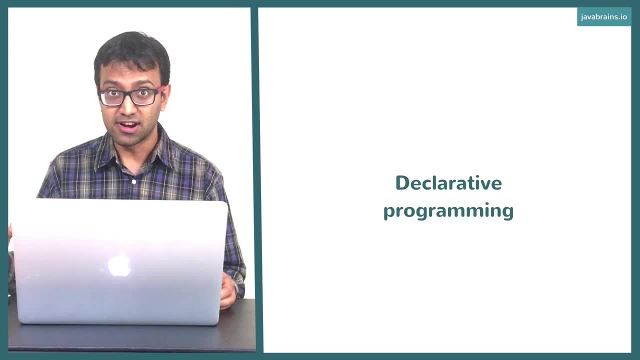 custom components and create the logic for it and then use it in multiple places, right? So here's one thing you need to remember, though: In all declarative code, you basically have to write the logic imperatively, right? So let's say, you're creating a date element, a custom date element. 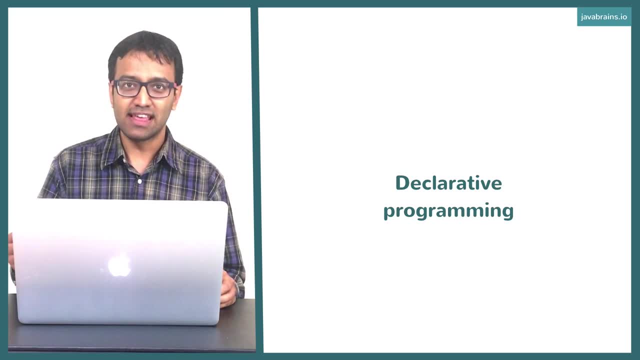 You're basically facilitating declarative programming by creating that element so that people can use it, But then you're going to have to create the logic for that element. But then the very first time you create and declare the element, you also have to define the logic and 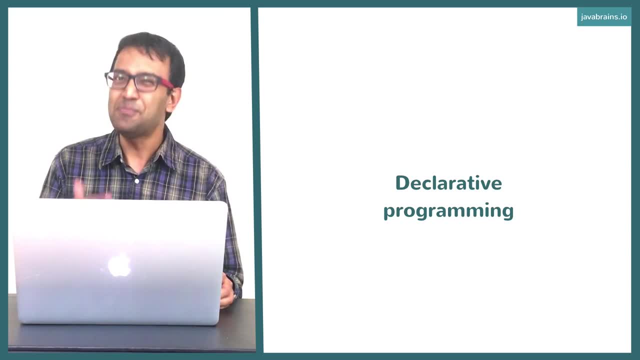 you have to define the logic imperatively. You have to define all the steps. Somebody has to write the code, but then, once that one person writes the code, it's available for others to use declaratively. right, I hope this makes sense. This is kind of like the central concept behind Angular. 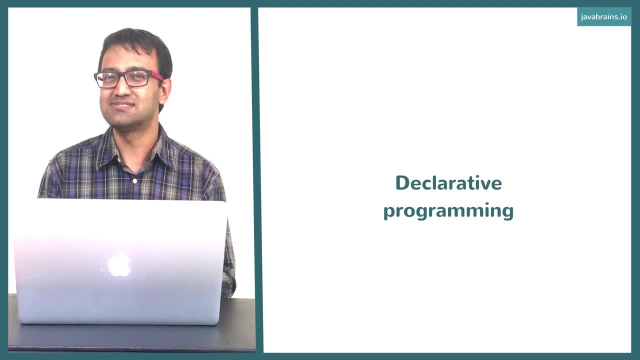 and not a lot of online tutorials kind of touch upon this concept, but this is fundamental in kind of understanding how to write code in Angular and understanding how to write good code in Angular. I would say So hopefully this makes sense. I definitely encourage you to kind of google the difference between these two declarative and 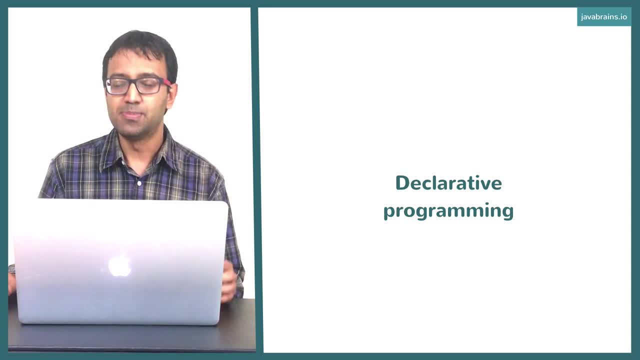 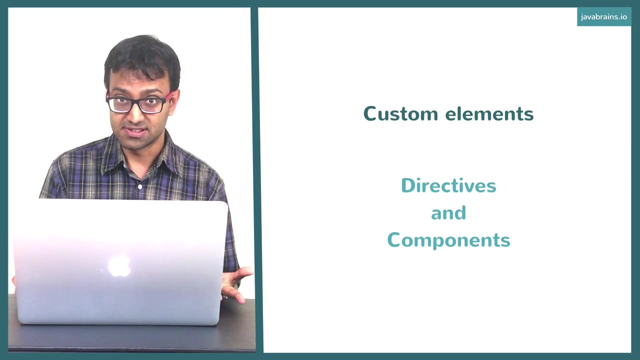 imperative and kind of research. that a little bit more if you're curious, But that's like the fundamental concept with Angular. You create those custom elements and then you use them in multiple places. These custom elements in Angular are called components or directives, Turns out there. 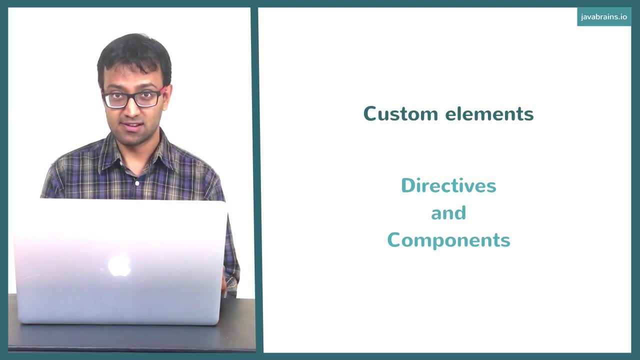 are two different ways of creating custom elements in Angular. One way of doing it is by creating what's called directives. Another way of doing it is by creating what's called components. This is one problem with Angular. For anything you want to do, there are multiple ways to do it. 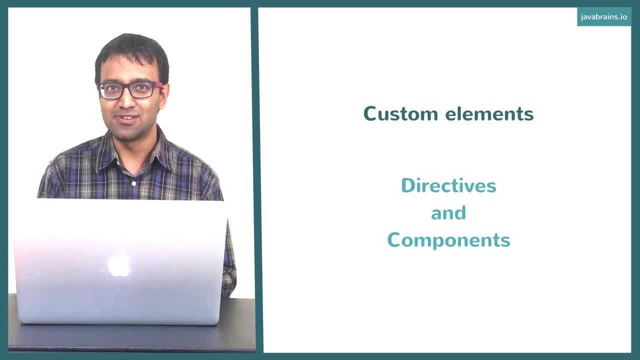 That's because of how old Angular is. It's been there for years now and there have been new ways of creating things, new features that have been introduced. So in a lot of things that you learn with Angular, there'll be multiple ways of doing the exact same thing. So it's important. 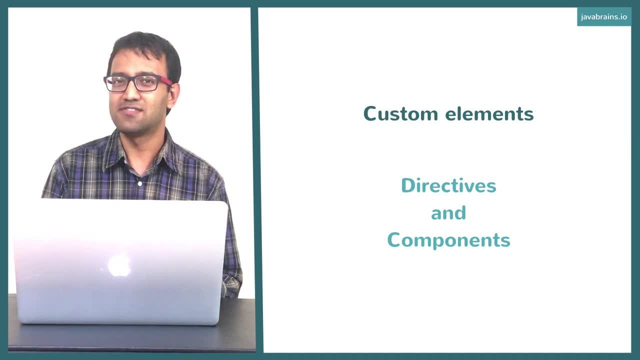 to understand the distinction and when to use what. I'll try to cover a lot of that in this course. So there are two ways of creating these custom elements. One is by creating directives, Another is by creating components. So some examples of some components you'd want to create. 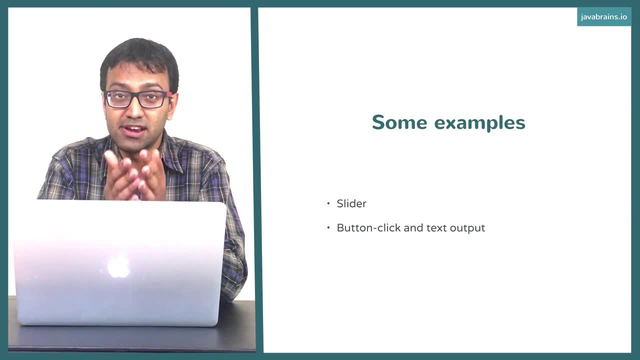 Something like a slider could be a custom element. You create a slider using a custom HTML tag. You can have a less than slider greater than You're extending HTML by creating your own slider element. Then you can use it in your code wherever you need a slider Or a button click and.